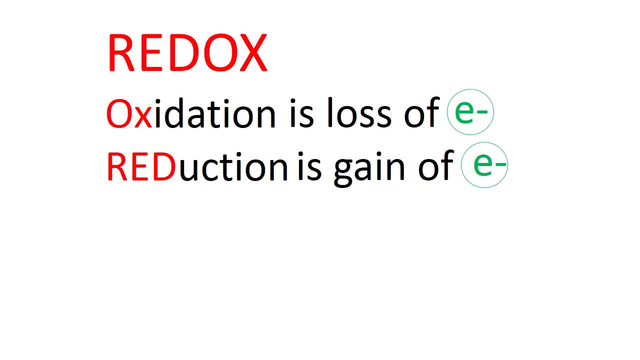 Something has to become reduced. Why do we call it reduction? Well, sometimes this is confusing. How does something gaining electrons become reduced? When you gain electrons, what happens? It becomes more, what More negative, And when you become more negative, your charge. 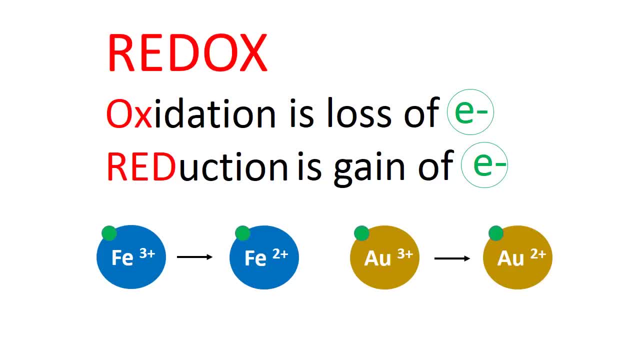 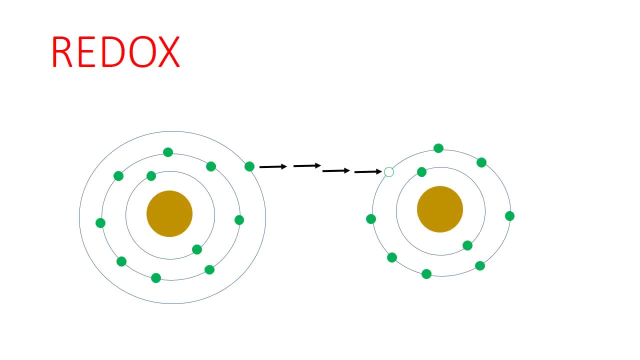 becomes more reduced or more negative. So from this you can see that an atom cannot become oxidized without another atom becoming reduced. These reactions are completely tied together. To help remember what the term reduction and oxidation mean, sometimes students will use the mnemonic oil rig. Oil means oxidation. 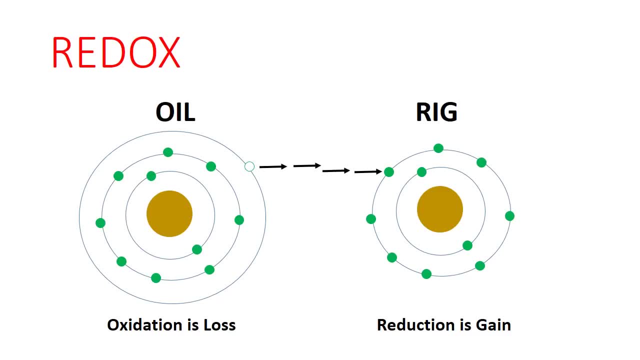 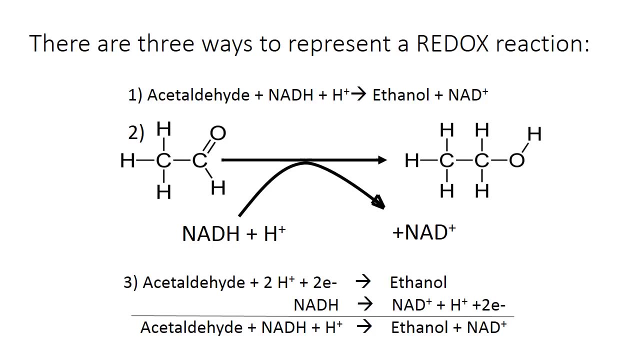 is loss, Rig means reduction is gain. There are three ways of representing redox reactions, which are shown here. This is the same reaction written in all three ways. The reactants are acetyl aldehyde, NADH and a proton. The products are ethanol nitrate and zinc. These reactions 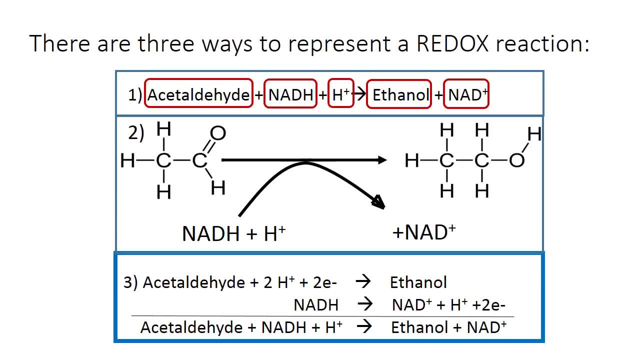 have been broken down into two half reactions. The top reaction here is the reduction half and the bottom reaction is the oxidation half. We know this because of where the electrons appear in the half reaction. If to form ethanol we need to add two electrons to acetyl aldehyde, 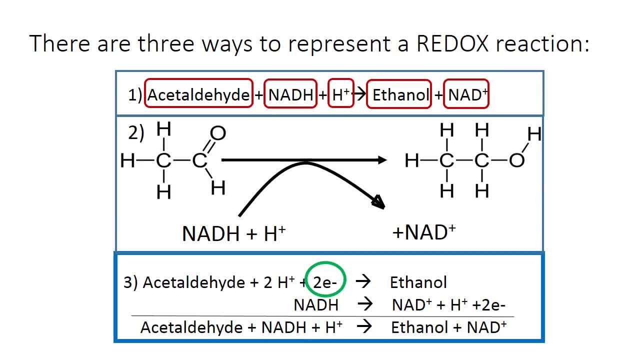 then we know that ethanol is the product of adding two electrons onto acetyl aldehyde And we know that reduction is gain of electrons. Let's look at the other two reactions: The oxidation, half reaction. If we look at the before and after, if we removed two electrons, 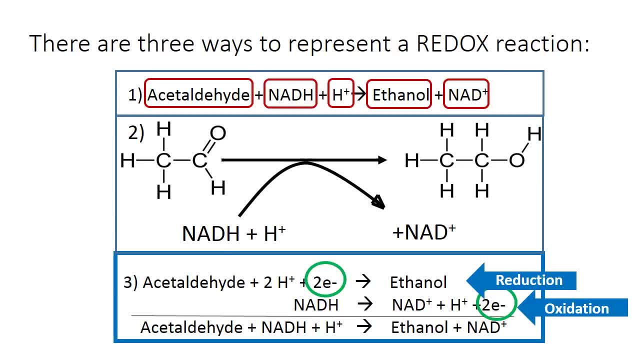 from NADH we produce NAD+. Loss of electrons is oxidation. Therefore, in this reaction we can say that ethanol is the reduced form, that acetyl aldehyde is the oxidized form of the carbon compound. NADH is the reduced form and NAD plus is the oxidized form of. 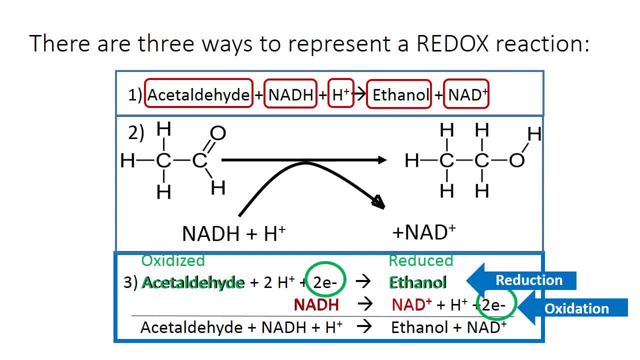 this compound, NADH, is really important in metabolism. You're going to see this in the next slide. In this example we can see this compound over and over again. This is an electron carrier. It moves electrons from one place to another in the cell. So when you see it as a reactant- 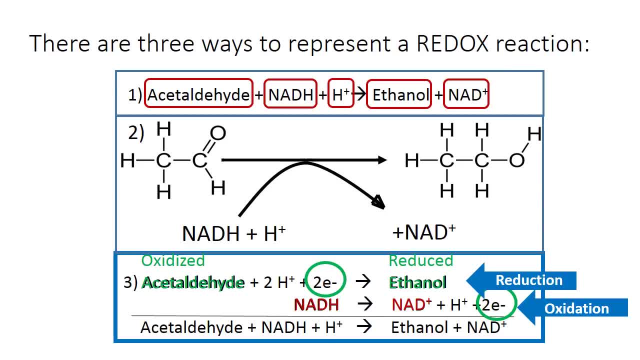 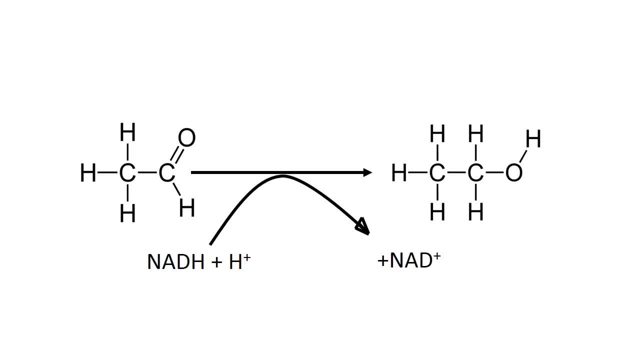 or a product of a reaction, you automatically know that it is a redox reaction. If we didn't have the half reactions, then we could take a look at the structure of the compounds to determine if they were oxidized or reduced. In biology we deal with a lot. 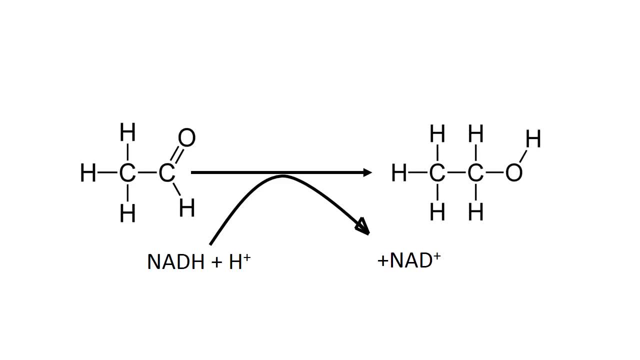 of metabolic reactions that oxidize or reduce carbon compounds. In this example, we can see that acetyl aldehyde has four carbon-hydrogen bonds, compared to that of ethanol, that has five carbon-hydrogen bonds. We know that electrons can move with hydrogen atoms, So when we compare, 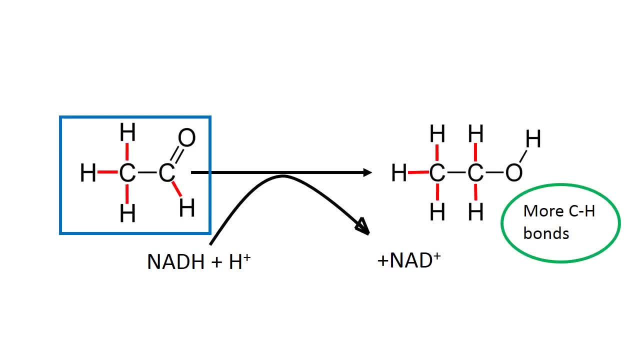 these two compounds, the one here with more carbon-hydrogen bonds is more reduced than the compound with less carbon-hydrogen bonds. But why did this happen? Why did electrons move from NADH onto acetyl aldehyde to form ethanol? This is not something that you're 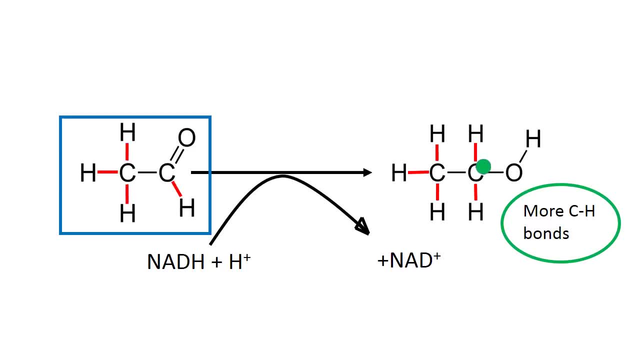 going to need to remember. This is not something that you're going to need to remember. You're going to need to memorize for every single metabolic reaction. There's a tool called a redox tower that we can use to predict the movement of electrons in biological reactions. 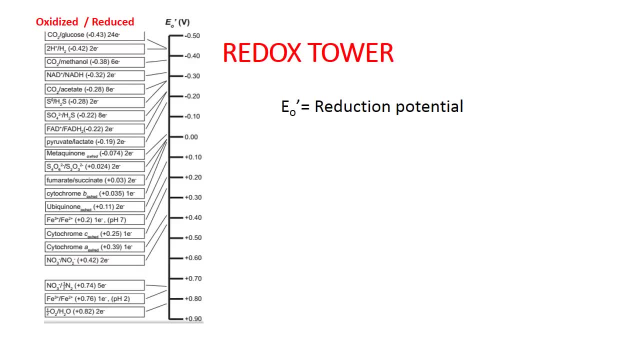 Here's the basic structure of a redox tower. We have a list here of half reactions and their E-value. This value is the reduction potential, which is the likeliness of a compound to gain electrons. The organization of the tower shows positive E-values at the bottom. 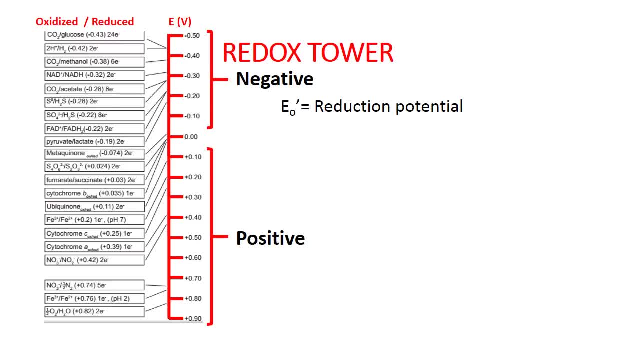 with negative E-values at the top. This means that the compounds at the bottom of the tower are more likely to gain electrons. when you compare one of these compounds to one at the top of the tower, You may also notice a slash on each line of the tower On the left-hand. 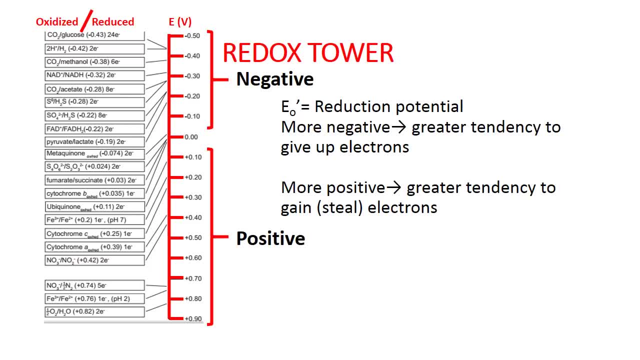 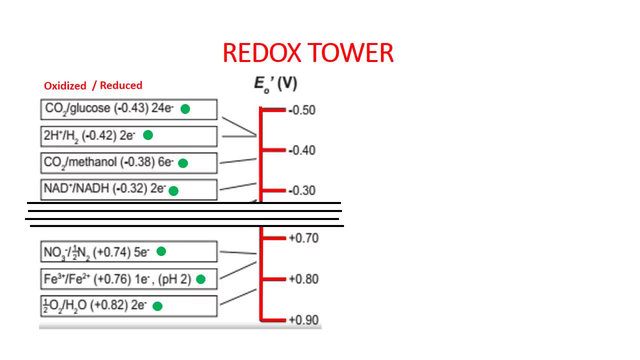 side of the slash is the oxidized form of the compound. The right-hand side is the reduced form of the compound. Let's take a closer look at the electrons moving from one compound to another. Let's take a closer look at the electrons moving from one compound to another. 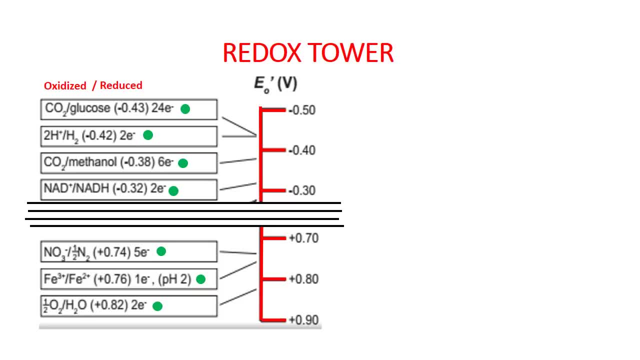 Let's take a closer look at the electrons moving from one compound to another. Using the redox tower, let's combine the two half reactions shown here: hydrogen gas and NAD+. When we combine two half reactions using the redox tower, we can answer several questions. 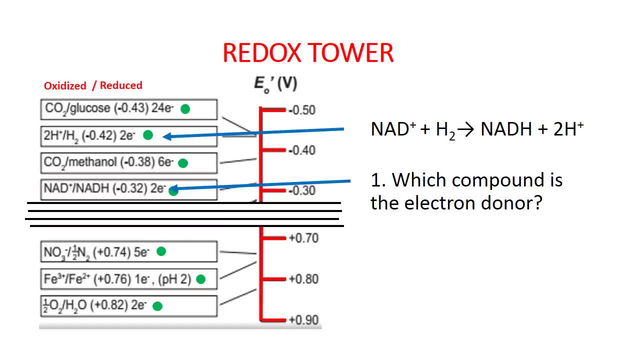 about the reaction. We can ask which compound is the electron donor and which is the electron acceptor. Using just the information in the tower, we can see that the NAD half reaction sits below hydrogen gas on the tower And compounds that sit lower on the tower are 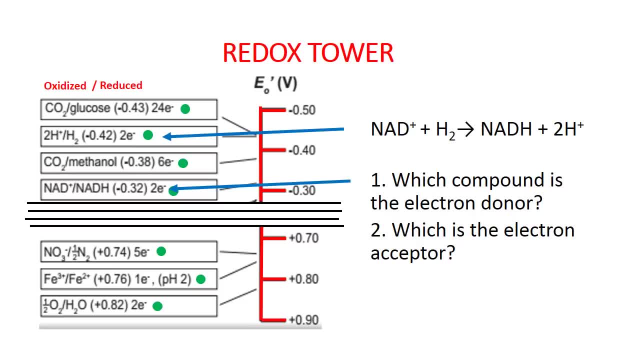 more likely to gain electrons. Therefore, the electron donor needs to be either hydrogen gas or the protons. From here you look at either side of the slash, the oxidized form and the reduced form of this compound. The reduced form has electrons. The oxidized form? 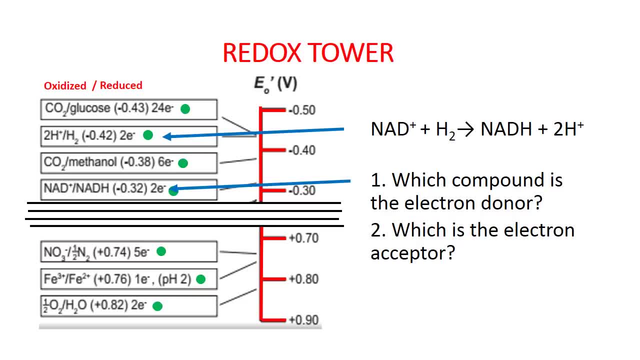 does not. Therefore, hydrogen gas will be the electron donor And this electron will fall down the tower and reduce NAD plus to form NADH. Let's look at one more reaction. This is the equation often used to represent the many reactions involved in central metabolism. First, let's find our two half reactions. 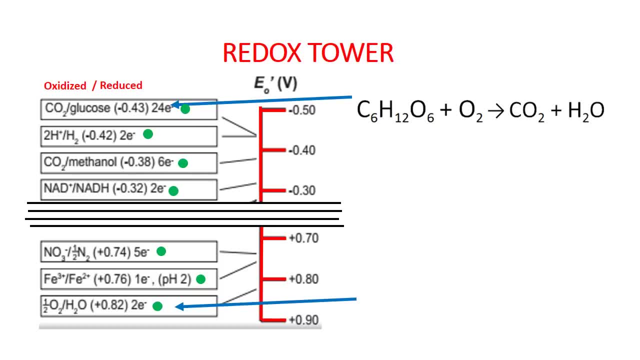 Glucose is here at the top and oxygen is here at the bottom of the this tower. Let's ask our questions again: Which compound is the electron donor and which is the electron acceptor? The glucose half reaction is above the oxygen half reaction. Therefore the reduced compound. 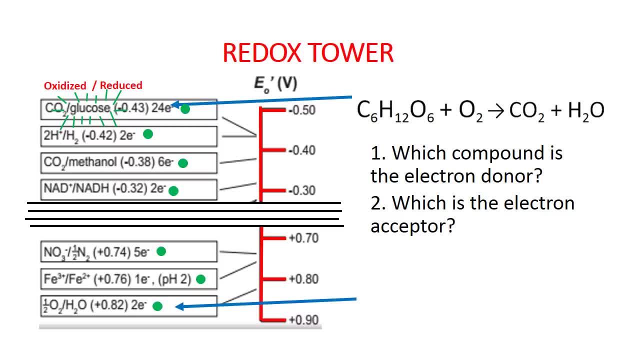 off the top half, reaction will act as our traces of carbon. OK, Let's look at the four electron donor. So when oxygen here accepts electrons from glucose, which oxygen wants to do, not just because it's at the bottom of the tower, but also 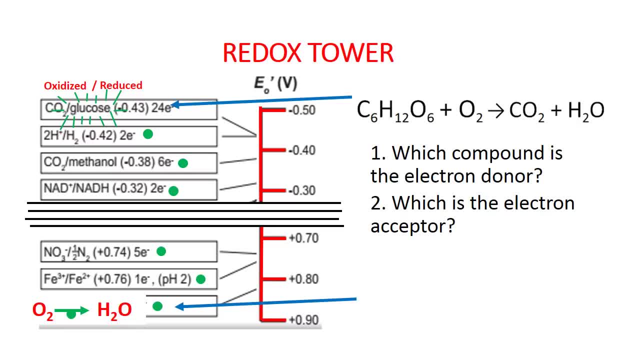 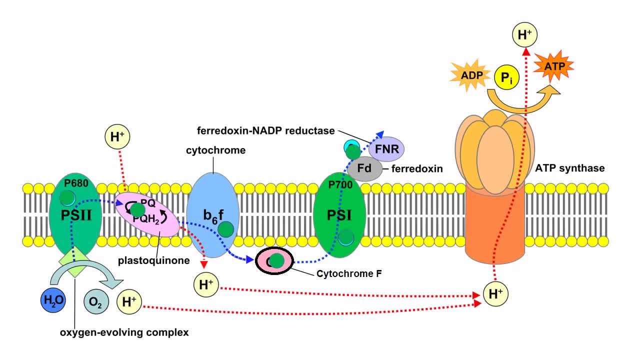 because it is below the glucose half reaction, it will become reduced forming water. There's one more element to redox towers that I want to discuss, and that is using a redox tower to predict the movement of electrons and electron transport chains. Here we're going to use the electron transport chain from 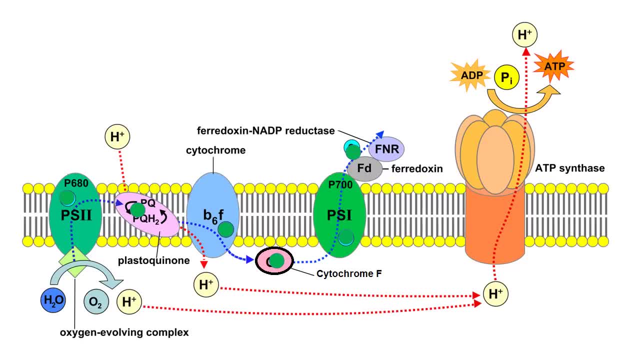 photosynthesis. Remember that electron transport chains exist inside of membranes because they are pumping hydrogen ions across the membrane in order to form a gradient, So light is going to hit photosystem II. This light energy changes form into chemical energy as it excites this electron. The excited 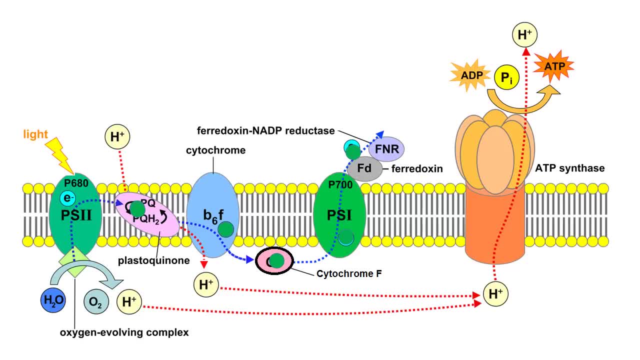 electron moves to plastoquinone, This reduces plastoquinone. This means that plastoquinone is a plastoquinone. This means that plastoquinone is a plastoquinone. must sit lower on the redox tower than the excited photosystem II. The electron 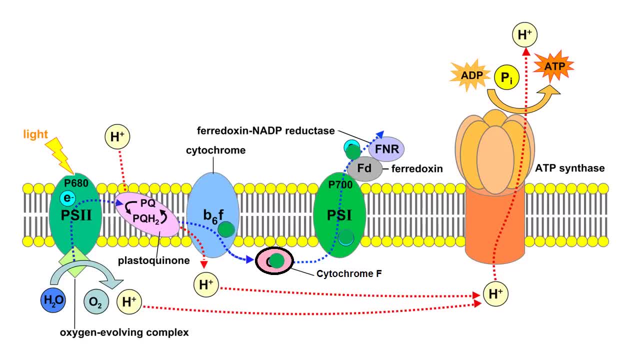 now moves from plastoquinone on to cytochrome B. In this transfer step, plastoquinone becomes oxidized and cytochrome B becomes reduced. So with each transfer in an electron transport chain it is actually a redox reaction. 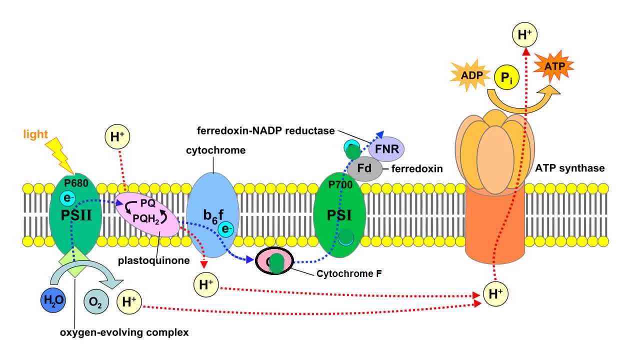 From cytochrome B the electron moves to cytochrome F and then finally on to photosystem I. At this point the electron is pretty low in energy. The energy has been used to pump protons across the membrane. So now in our story. 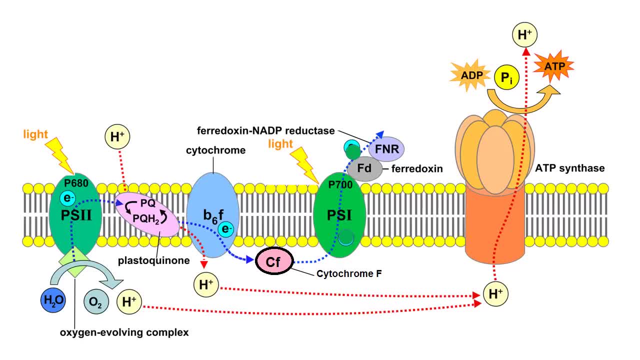 of this electron photosystem. I will now need to absorb light energy in order to excite this electron. The light energy will be converted to chemical energy as the electron becomes excited and leaves the photo center on to ferridoxin. Ferridoxin will then lose the electron to FNR and FNR will eventually dump the 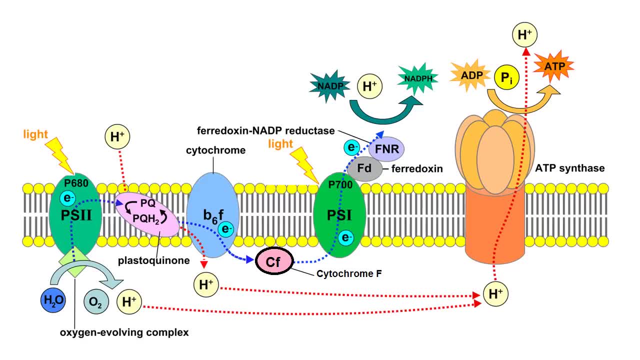 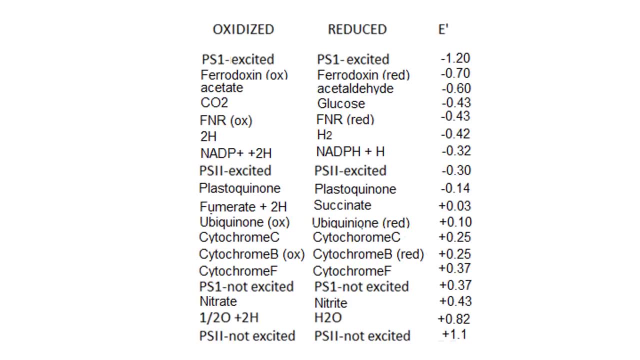 electron on to NADP. So here's that information written in table form. We start with an unexcited photosystem II. It absorbs light to form the excited state. Once it absorbs this light, the photosensor now becomes a very powerful electron donor. 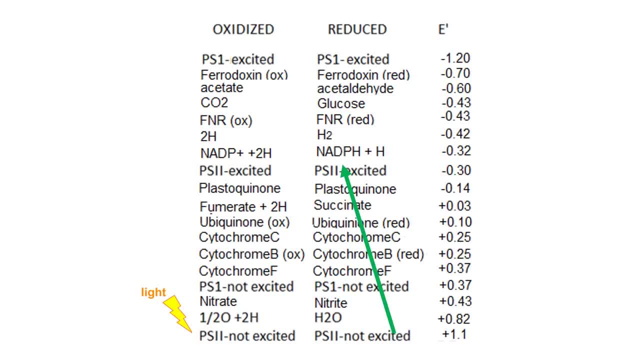 We know that because the redox potential has become very negative and it sits higher on the redox tower. We can follow the same steps as in our picture on the previous slide all the way down to photosystem I. You can see that the energy in this electron has greatly diminished once it reaches photosystem. 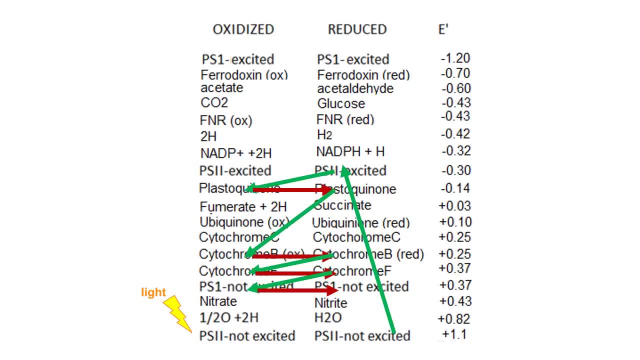 I, because photosystem I sits low on the tower in the unexcited state. The compounds that accept low energy electrons sit lower on the tower in general because they have to have a very strong reduction potential to accept electrons when the electron is very low in energy. But that is soon fixed when photosystem I absorbs light. 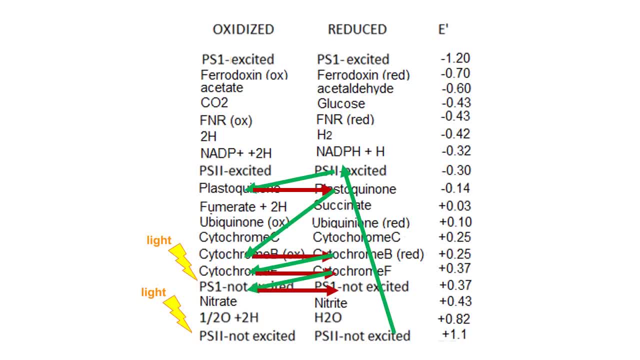 But that is soon fixed when photosystem I absorbs light Photosystem, I is now in the excited state and we can follow this electron all the way down to the final electron acceptor, NADP, to form NADPH. We have now 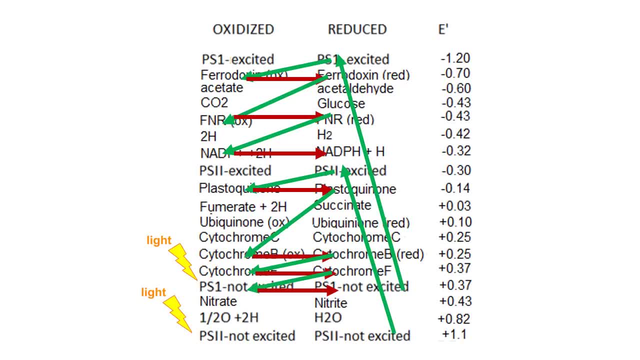 followed this electron from the very beginning of the electron transport chain on to NADPH. But where did this electron come from in the first place? Once we have excited an electron from photosystem II, it ends up on NADPH. Therefore, photosystem II is now in the oxidized state and can no longer. 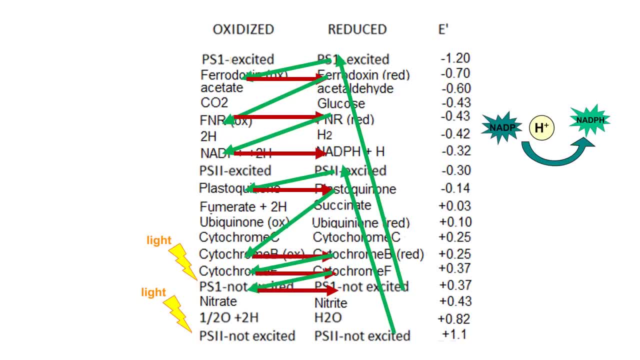 absorb light energy to excite an electron. So my question now is: what on this tower would be a good donor for photosystem II? which compound here can donate an electron? This is a typical test question for this class. Can you, using a, 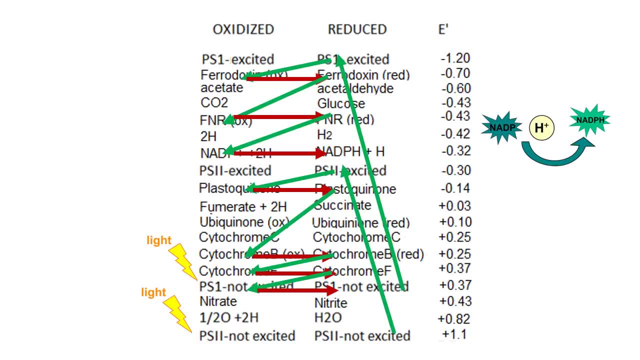 Redox tower, pick out a good electron donor for photosystem II. The answer is basically anything that sits above photosystem II in the tower. In nature we know that photosystem II has the power to pull electrons off of water, and water sits above photosystem II. How do you know that photosystem II does? You could know that photosystem sees the energy being absorbed- light energy- by 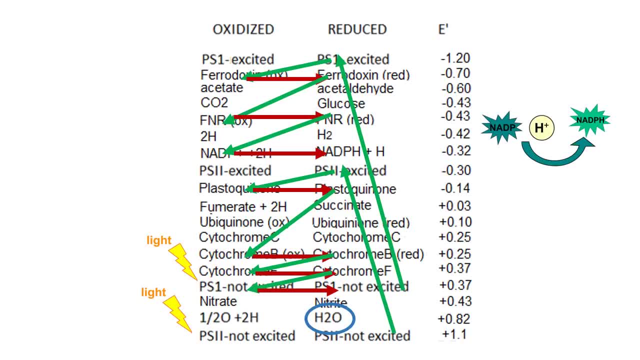 absorbing electrons. in some of the electrons that series��, ha cuộcBAef to 이�比子 f' bisog难 of Photosystem II on the tower. Other potential donors on this tower shown here are also possible, but the drop from, say, hydrogen gas to Photosystem II is relatively large. This huge of a drop could. 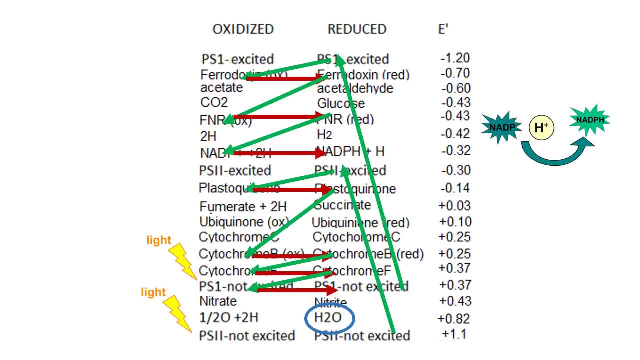 be potentially disastrous for the cell. that energy released can form a lot of heat or a little miniature explosion in the cell, So drops are usually kept small. as you can see by all the steps between each photosystem we have highlighted on this table, 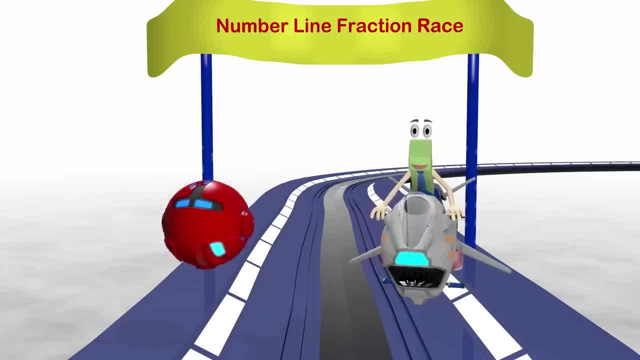 Hey kids, thanks for joining me today. I am here at the number line fraction race with my friend, Mr Robot. We are racing each other While we do a few practice runs. can you guys learn about fractions on a number line? Great Okay, Mr Robot, on your mark, get set hey. 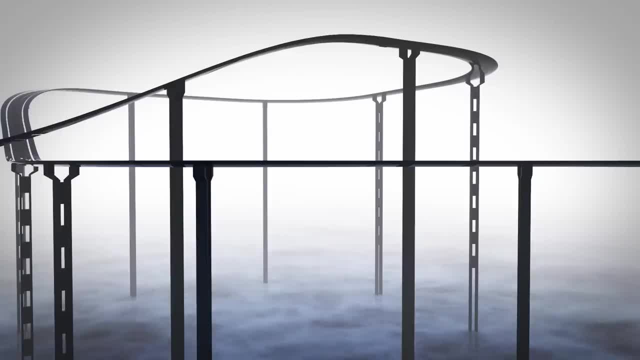 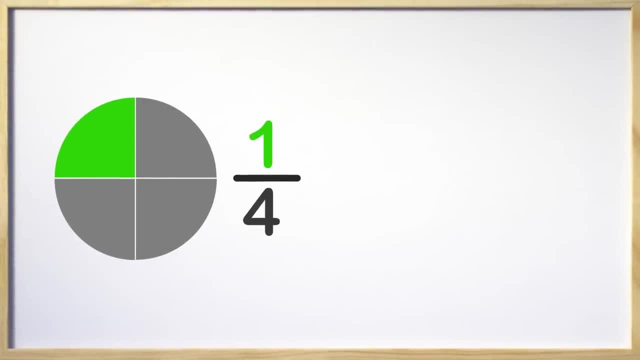 I didn't say go yet. To start off, let's review some concepts about fractions. Here we have a fraction of one-fourth. A fraction is a part of a whole or a part of a group. The numerator is the number on top and shows the parts we are talking about In this case.